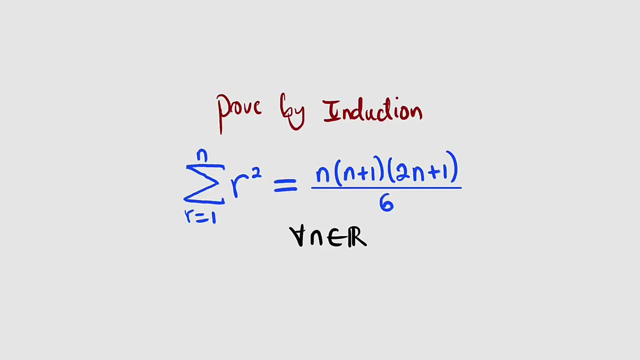 Hello, good day viewers, Still on mathematical induction. In this tutorial we want to prove that the summation of r, squared r, from 1 to n is exactly the same as n multiplied by n plus 1, multiplied by 2n plus 1 divided by 6, for all n in the set of real numbers. Okay, as you all know, 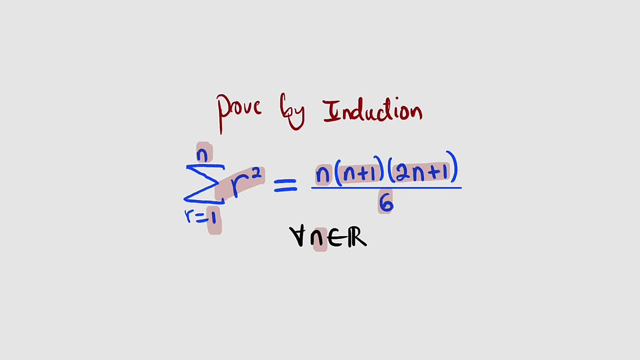 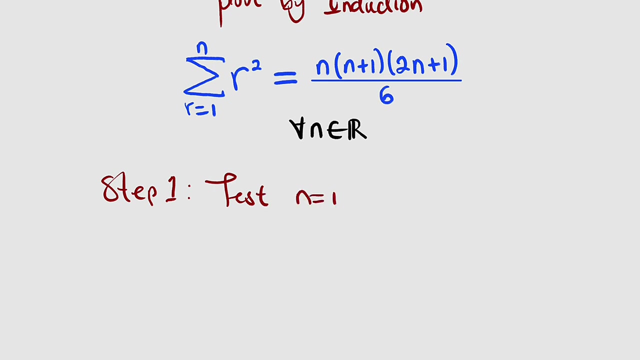 we have three basic steps. The first step is to test for n equal to 1, to see whether the left and right hand side are exactly the same. So let's start. So, step one: we want to test for n equal to 1.. Therefore, we have summation of r squared r from 1 to 1, which is equal to 1 multiplied by. 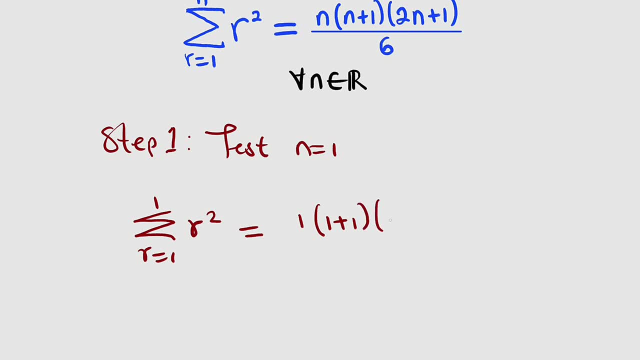 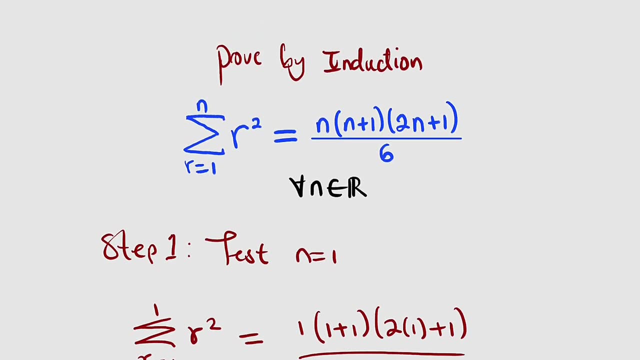 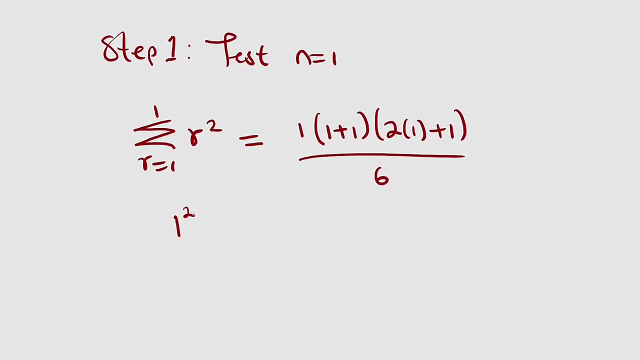 1 plus 1 multiplied by 2, multiplied by 1 plus 1 divided by 6.. We have just substituted n equal to 1 from left to right. So from the left hand side we have a single term: 1 squared substituted r, equal to 1.. And to the right hand side, we have 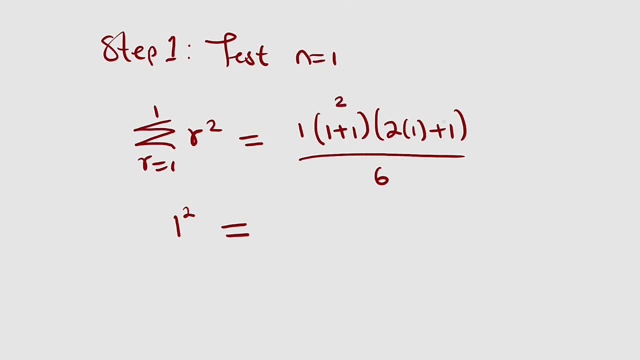 from this bracket, we have 1 plus 1, equal to 2.. From this bracket, we have 2 times 1, 2 plus 1, 3.. And we have 1 outside here. 1 times 2 times 3 is 6. 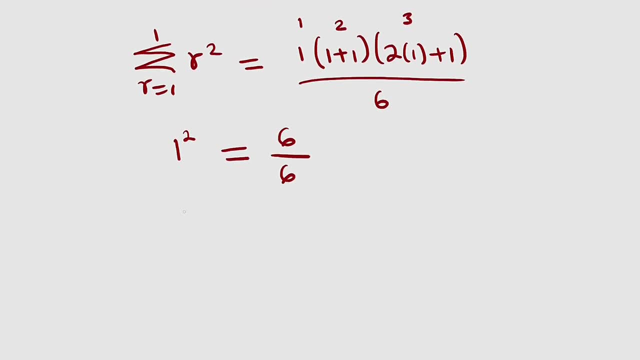 divided by 6.. From the left hand side we have 1 squared 1.. And to the right hand side we have 6 divided by 6, equal to 1.. So we have seen that 1 is true in the set of real numbers. So in the second step we want to also 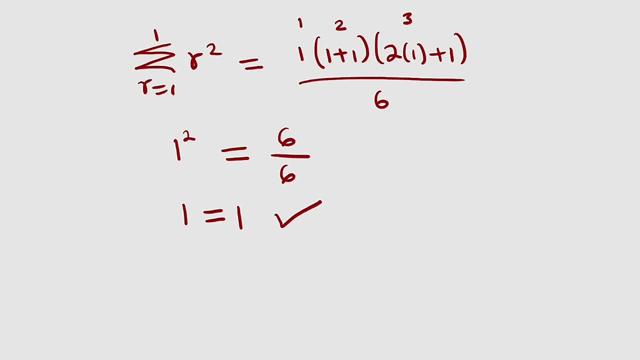 assume a certain value in the set of real numbers will be true. So we are going to set n equal to k, for which k belongs to the set of real numbers. So second step, Step 2.. We want to assume n equal to k is true. So what we have is the summation of r squared r from 1 to k. 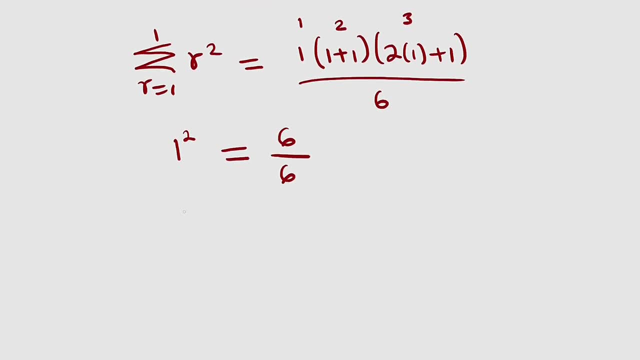 divided by 6.. From the left hand side we have 1 squared 1.. And to the right hand side we have 6 divided by 6, equal to 1.. So we have seen that 1 is true in the set of real numbers. So in the second step we want to also 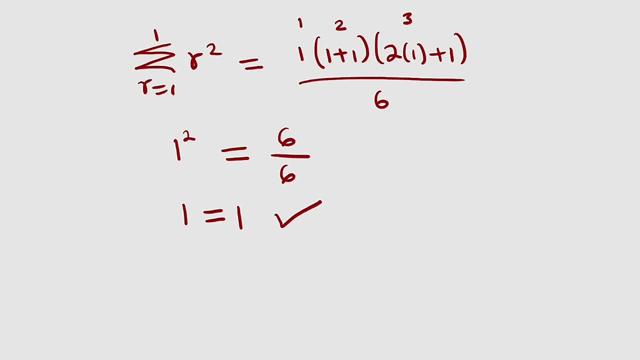 assume a certain value in the set of real numbers will be true. So we are going to set n equal to k, for which k belongs to the set of real numbers. So second step, Step 2.. We want to assume n equal to k is true. So what we have is the summation of r squared r from 1 to k. 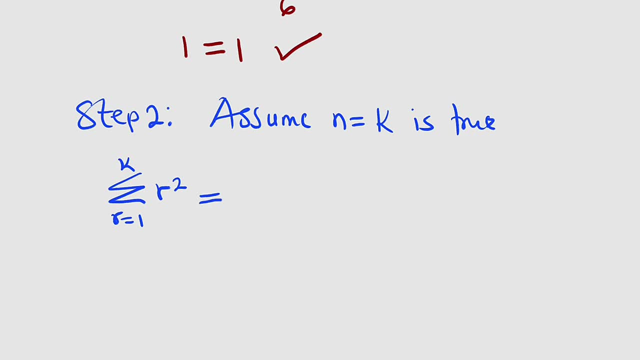 this time around- And this is equal, to remember, to right hand side, we have n, but we are going to replace it with k multiplied by n plus 1, k plus 1.. So this is the summation of r squared r, from 1 to k. 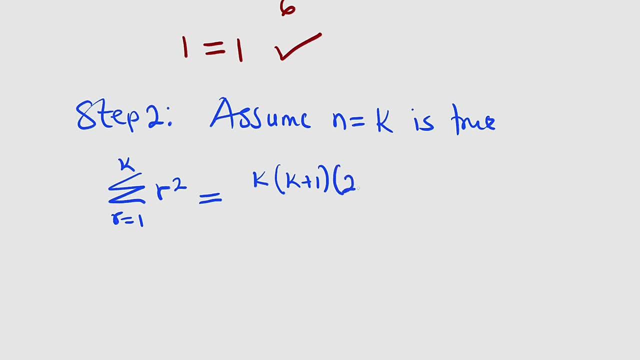 So we have 1 squared n plus 1, multiplied by 2n plus 1, 2k plus 1.. All of this divided by 6.. So we want to assume that this is true. Before we continue, let me break this down. 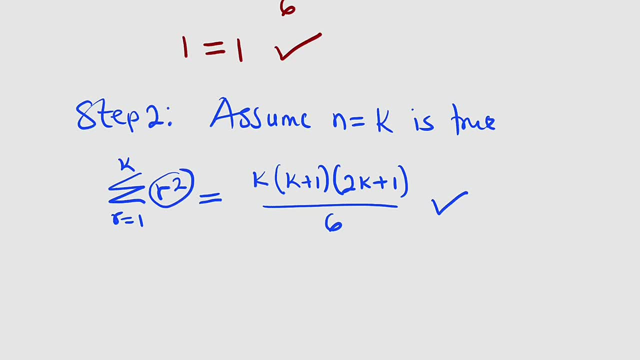 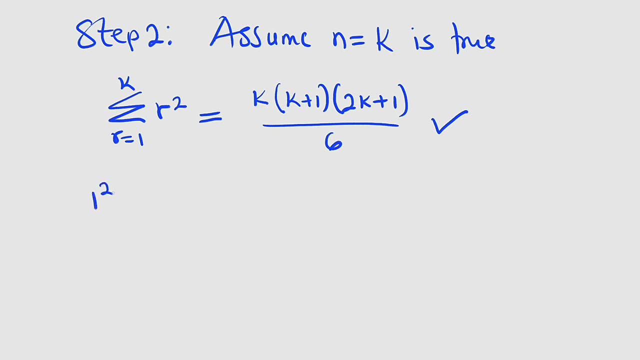 Remember, summation means you should be at a series of this. So if the two things are equal to 1 after k. So we have the first term, 1 squared, The second term, 2 squared, The third term, 3 squared, The fourth term, 4 squared, The fifth term, 5 squared. 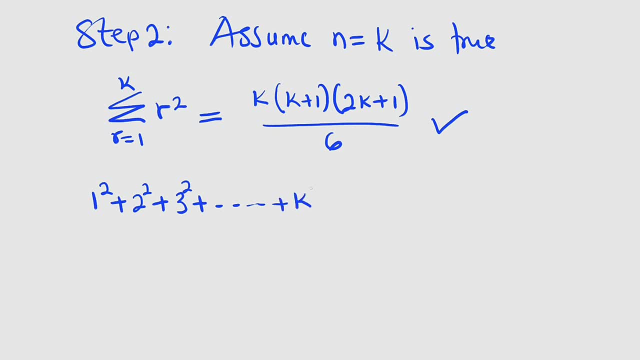 The sixth term, 6 squared. The seventh term, 7 squared Plus. you keep on adding these terms after the last term, k squared, And it will still be equal to k multiplied by k plus 1, multiplied by 2k plus 1, all divided by 6.. 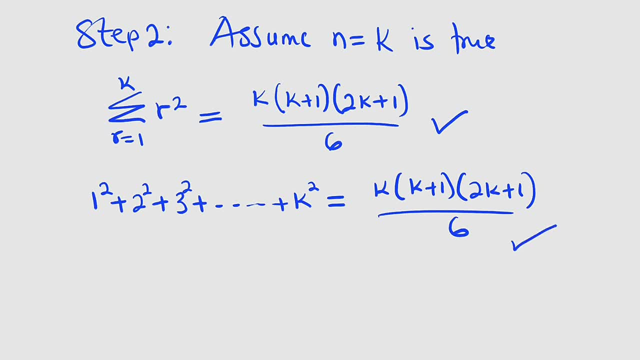 So we want to assume that this statement is true. So if it is true, in the last step we want to prove k plus 1 will also be true. What does that mean? It means any value you take in the set of real numbers. if it is true, the next term will also be true. 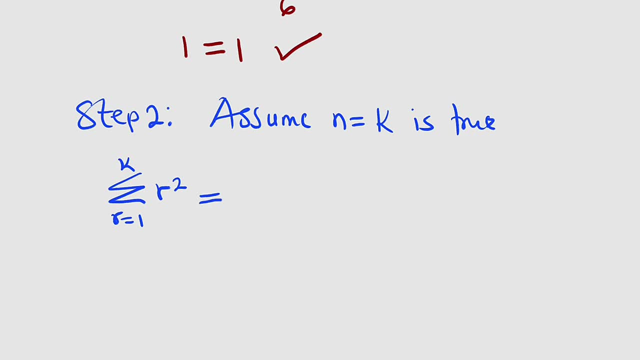 this time around- And this is equal, to remember, to right hand side, we have n, but we are going to replace it with k multiplied by n plus 1, k plus 1.. So this is the sum of r squared r from 1 to k. 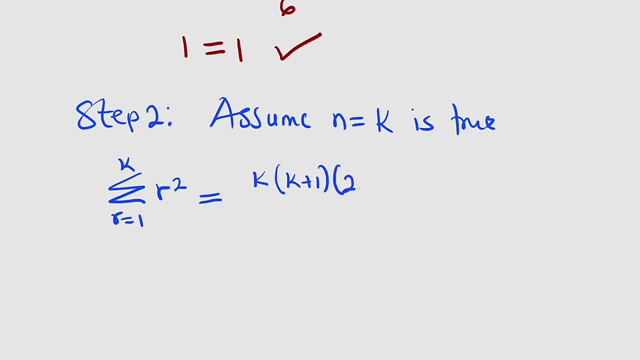 So we want to assume that this is true. Before we continue, let me break this down. Remember, summation means you should be at a series of this. So if the two things are equal to 1 after k, So we have the first term, 1, squared, The second term, 2, squared, The third term, 3.. 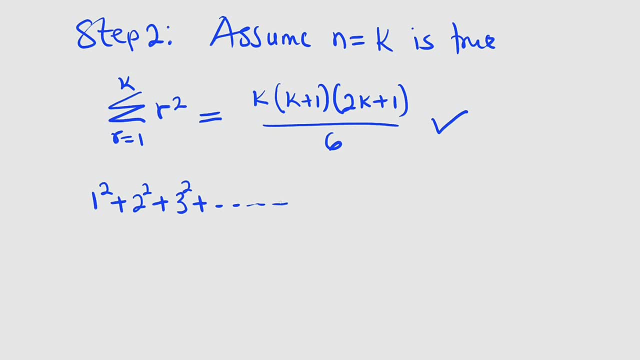 The third term, 4 squared Plus. you keep on adding these terms after the last term, k squared, and it will still be equal to k multiplied by k plus 1, multiplied by 2k plus 1 or divided by 6.. So we want to assume that this statement is true. 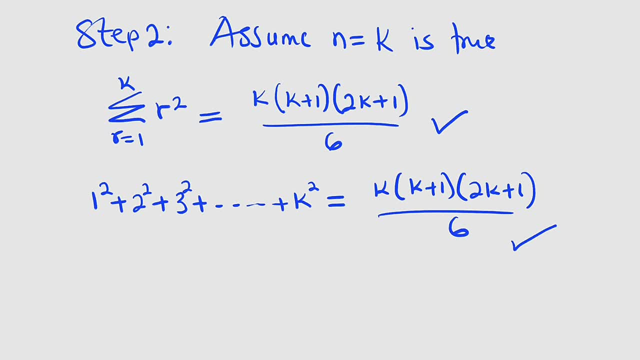 So if it is true in the last step we want to prove, k plus 1 will also be true. What does that mean? It means any value you take in the set of real numbers. if it is true, the next time will also be true. 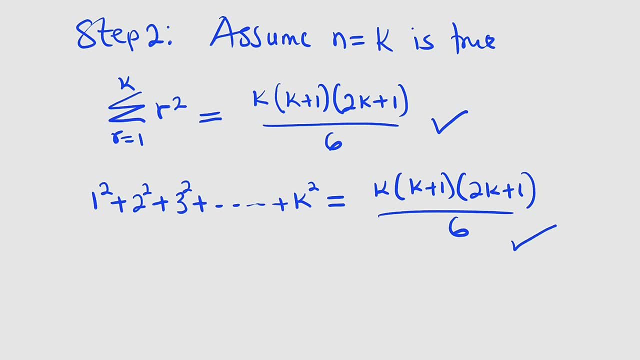 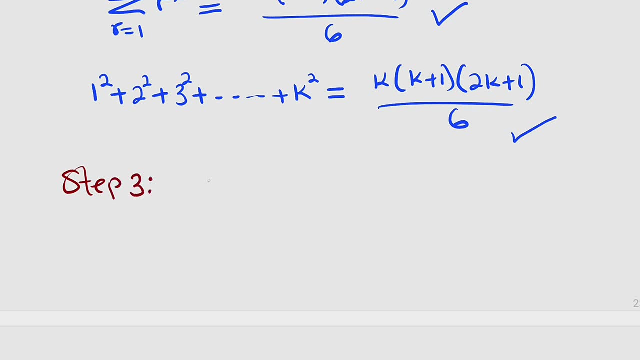 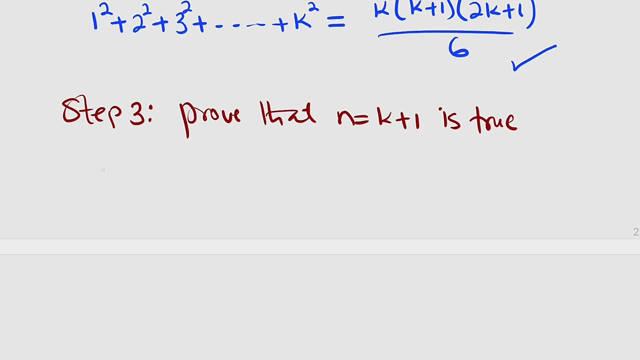 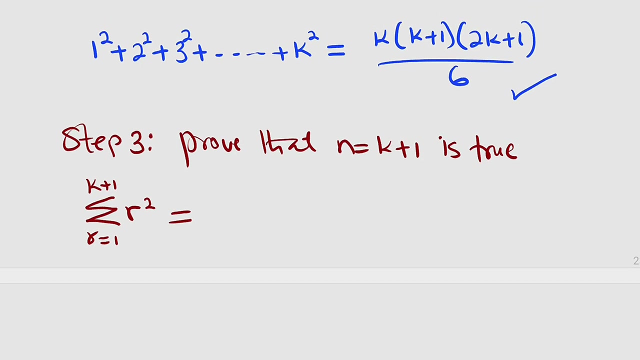 If 6 is true, 7 will be true. That is what it means. So step 3.. We want to prove that n equal to k plus 1 is true. So we are going to have a summation r, squared r from 1 to k plus 1, and this is equal to. wherever we have n, we are going to substitute it with k plus 1.. 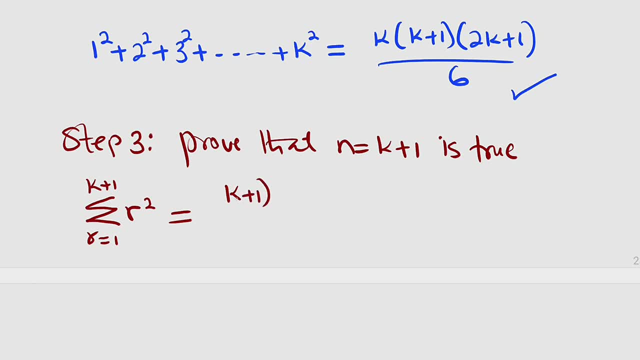 So we have k plus 1 multiplied by n plus 1, that is k plus 1, also plus 1.. Then we multiply it by 2k, 2n plus 1, that is 2 multiplied by k plus 1, for which k plus 1 is equal to n plus 1.. 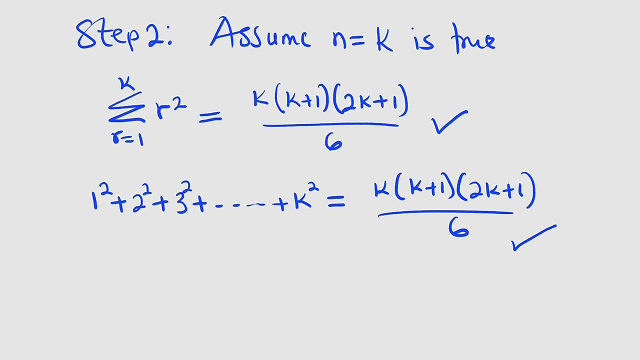 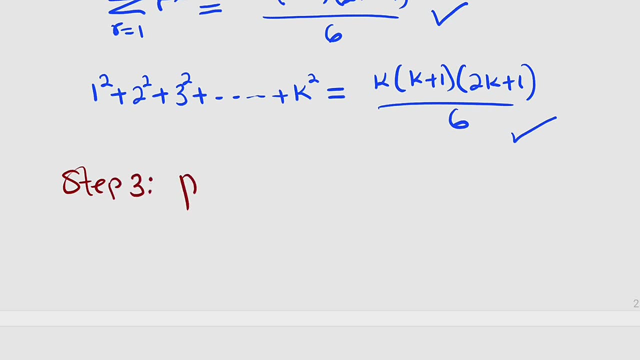 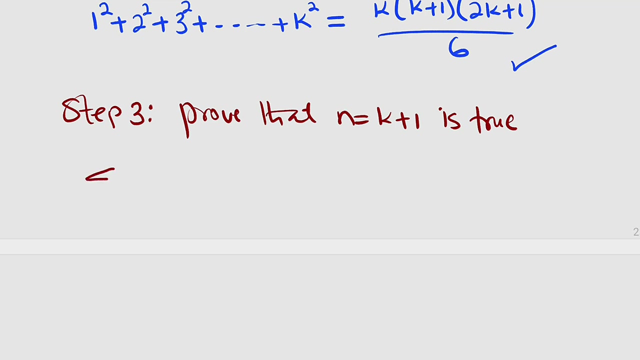 If 6 is true, 7 will be true. That is what it means. So step 3.. We want to prove that n equal to k plus 1 is true. So we are going to have a summation r, squared r, from 1 to k plus 1.. 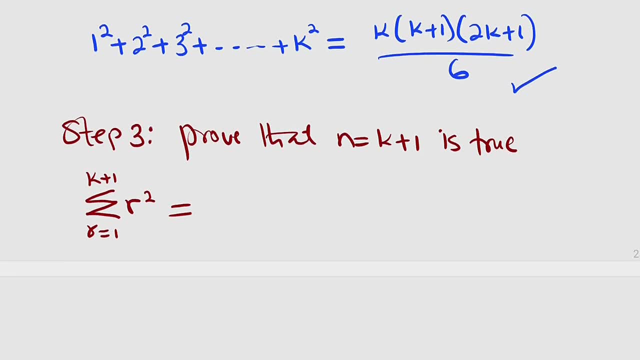 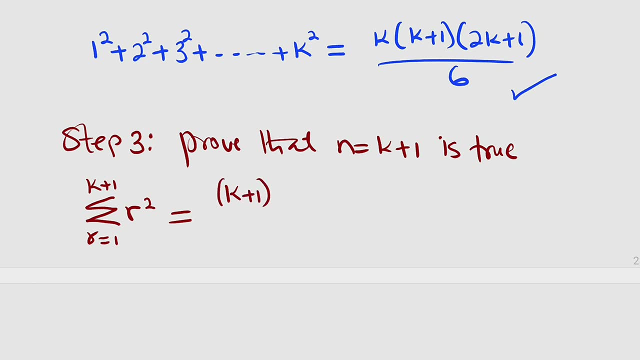 And this is equal to. wherever we have n, we are going to substitute it with k plus 1.. So we have k plus 1 multiplied by n plus 1, that is k plus 1, also plus 1.. Then we multiplied by 2n plus 1, that is 2 multiplied by k plus 1, for which k plus 1 is equal to n plus 1.. 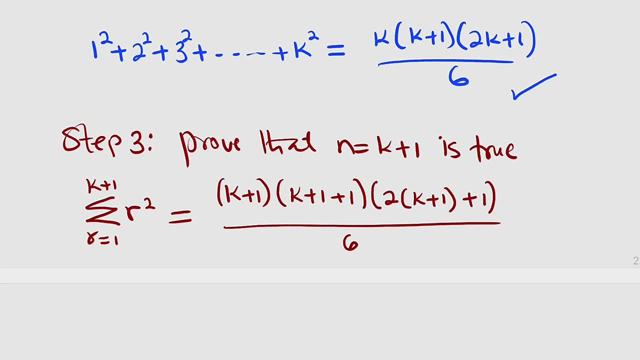 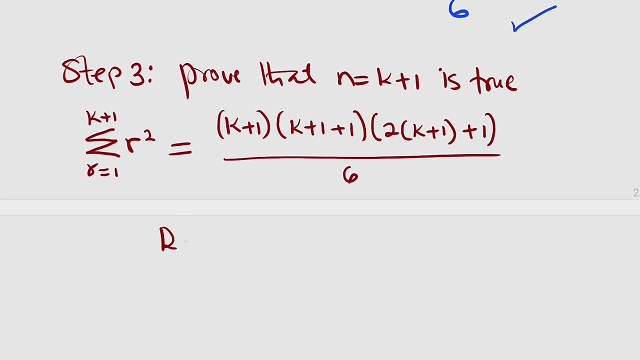 The whole of this divided by 6.. Let me first of all simplify the right hand side before coming back to the left hand side, The right hand side. from here you can see we have 1 plus 1 equal to 2.. So we have k plus 1 multiplied by k plus 2.. 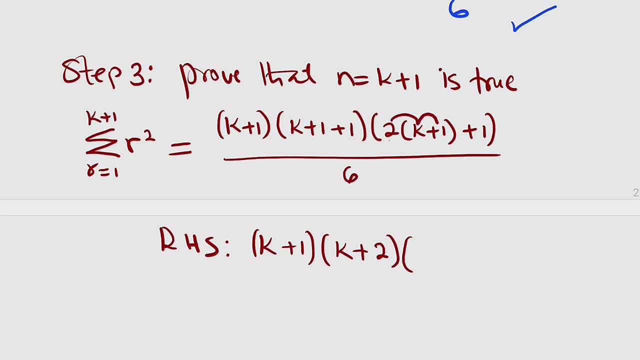 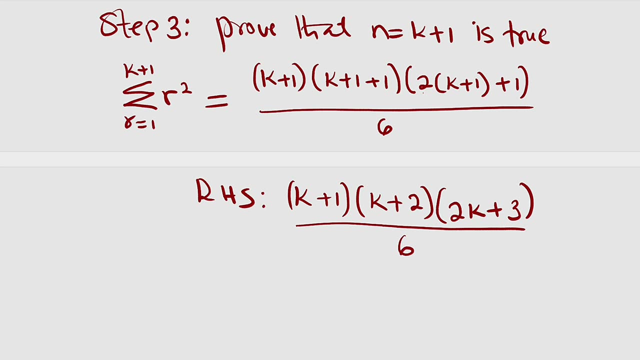 And the other factor: if you distribute 2 here, you are going to obtain 2k plus 2 plus 1, that is, 2k plus 3.. The whole of this divided by 6.. So this is what we have to the right hand side. 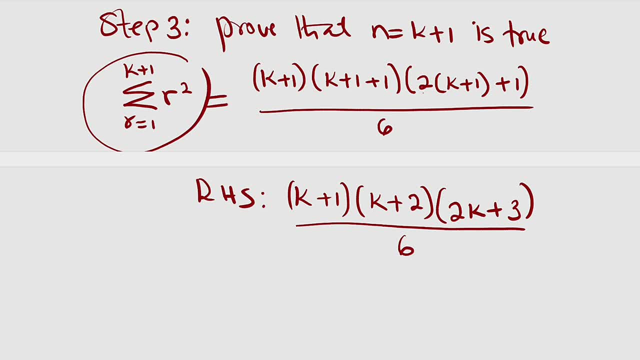 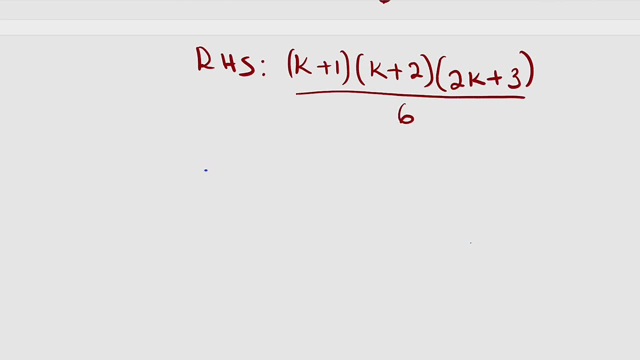 Now let us simplify the left hand side and see whether we are going to get the same thing. What we have to the left hand side is the summation of r squared r from 1 to k plus 1.. If you expand this, you are going to get 1 squared plus 2 squared plus. 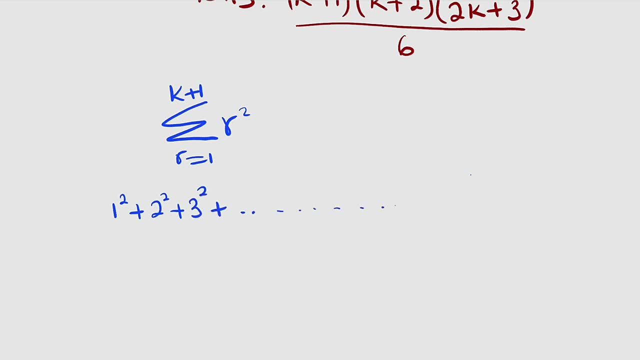 If you keep adding these terms, you are going to get to the last term, which is k plus 1.. All squared, But remember that the term before the last term is k, because k plus 1 is the next term after k, So we can add it here. 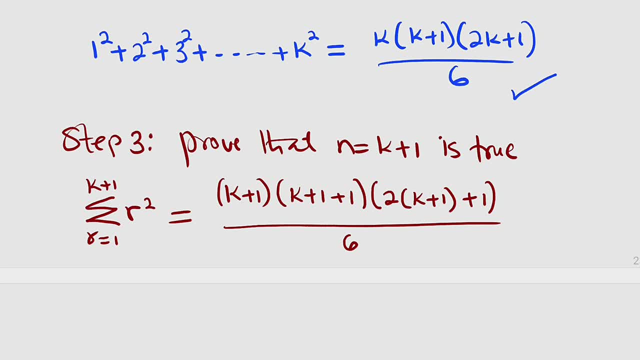 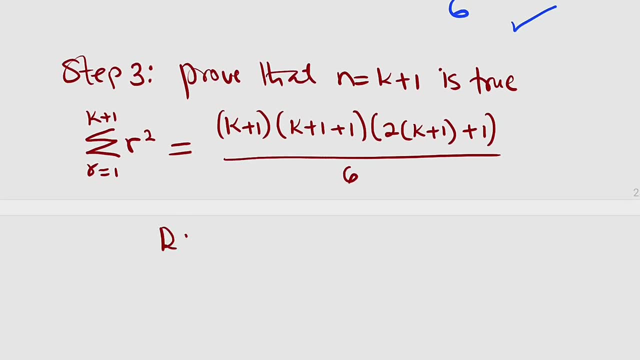 The whole of this divided by 6.. Let me first of all simplify the right hand side before coming back to the left hand side, The right hand side. from here you can see we have 1 plus 1 equal to 2. So we have k. 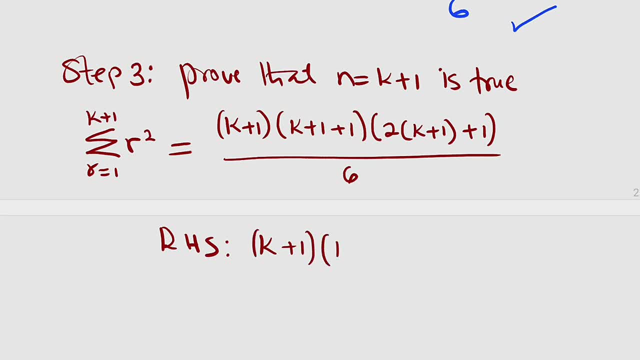 Plus 1, multiplied by k plus 2 right And the other factor. if you distribute 2 here, you are going to obtain 2k plus 2 plus 1, that is 2k plus 3.. 2k plus 3.. 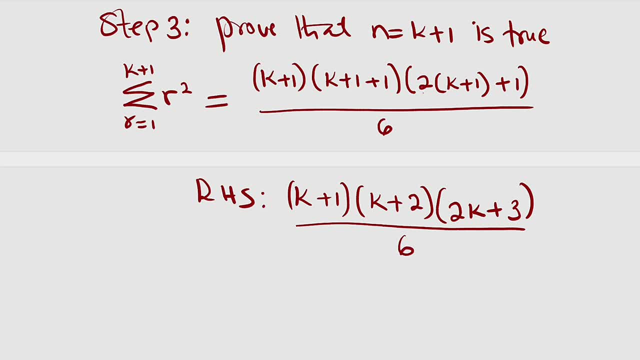 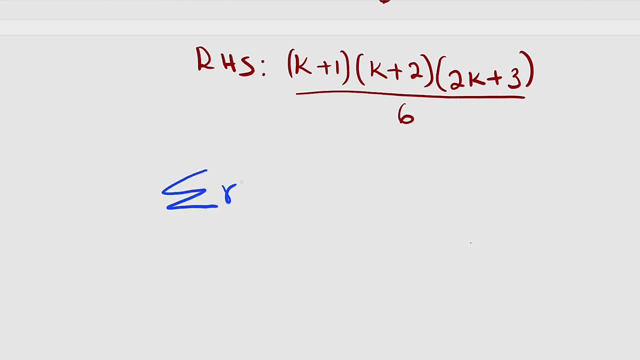 The whole of this divided by 6.. So this is what we have to the right hand side. Now let us simplify the left hand side and see whether we are going to get the same thing. What we have to the left hand side is the summation of r squared r, from 1 to k plus 1.. 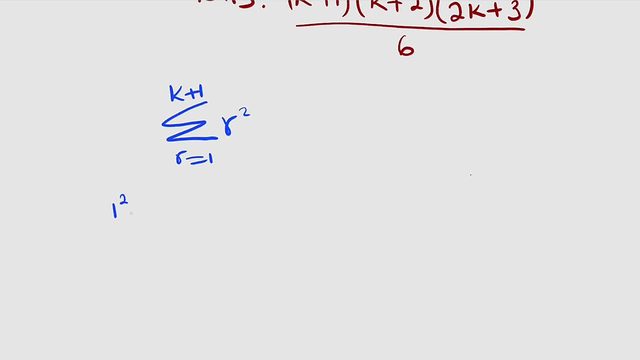 If you expand this, you are going to get 1 squared plus 2 squared plus. If you keep adding these terms, you are going to get to the last term, which is k plus 1 all squared. But remember that the term before the last term. 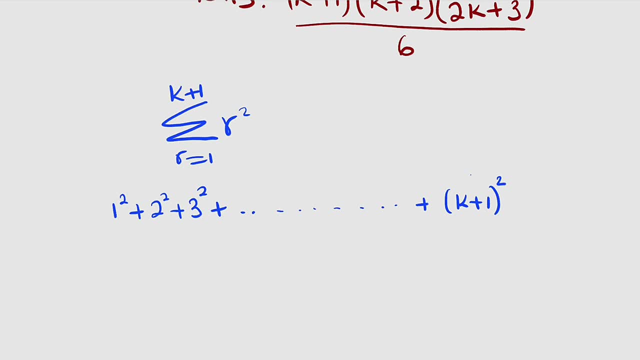 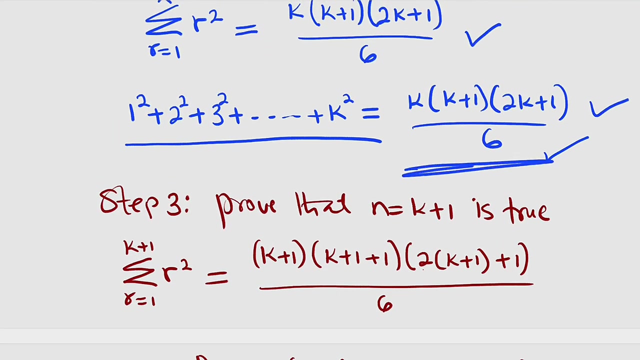 Is k, Because k plus 1 is the next term after k, So we can add it here: k squared. One thing you should observe is that we have this previously, Which is exactly equal to the right hand side here: k multiplied by k plus 1, multiplied by 2k plus 1 divided by 6.. 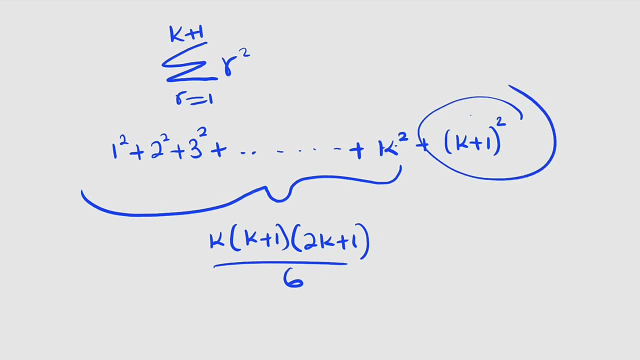 Which we are going to replace here. But we still have another term, which is k plus 1 all squared. k plus 1 all squared. To rationalize it, you can divide it by 6 or multiply it by 6, just to have common denominators. 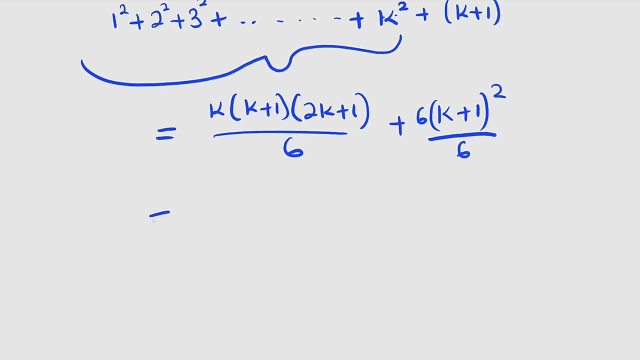 Now let us add denominators together. This will give us k multiplied by k plus 1, multiplied by 2k plus 1.. Then plus 6.. Multiplied by k plus 1, all squared, the whole of this divided by 6.. 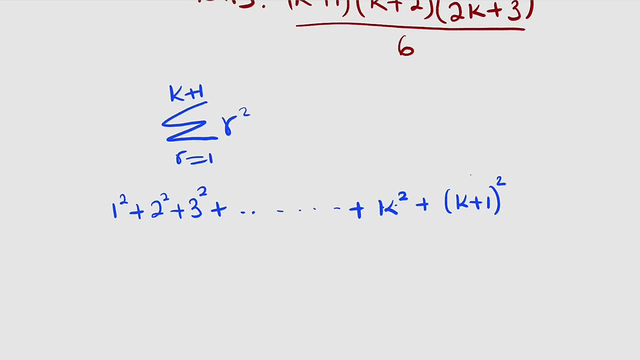 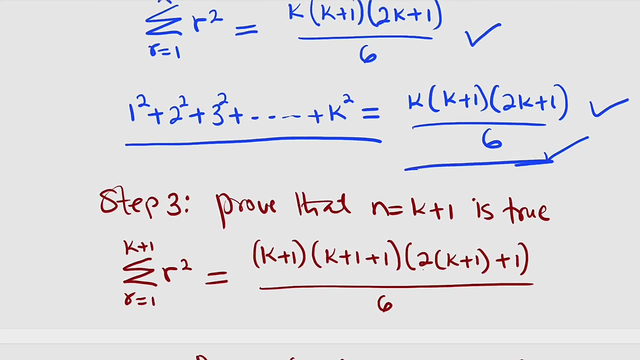 k squared. One thing you should observe is that we have this previously, Which is exactly equal to the right hand side here: k multiplied by k plus 1.. Plus 1 multiplied by 2k plus 1 divided by 6., Which we are going to replace here. 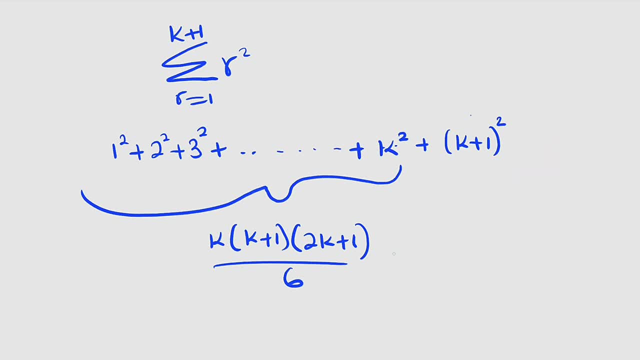 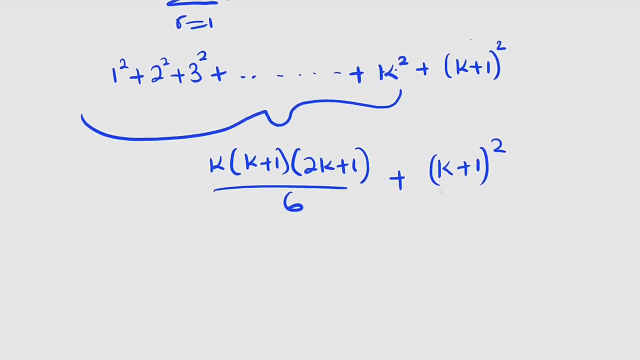 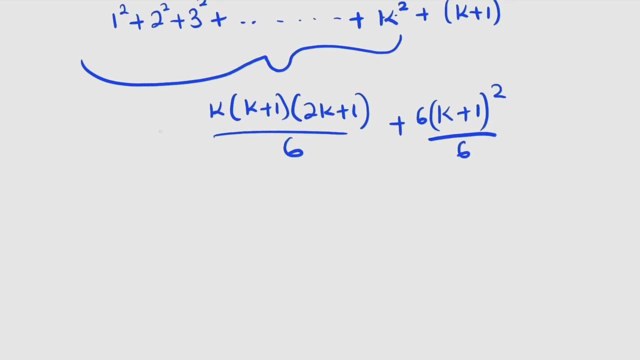 But we still have another term, which is k plus 1 all squared. k plus 1 all squared. To rationalize it, you can divide it by 6 or multiply it by 6, just to have common denominators. Now let us add denominators together. 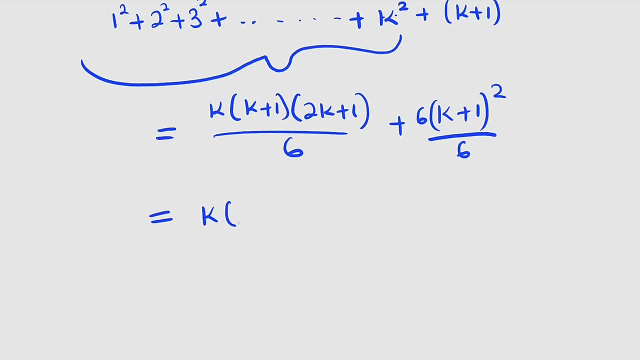 This will give us k multiplied by k plus 1, multiplied by 2k plus 1.. Then plus 6 multiplied by k plus 1. all squared, The whole of this divided by 6.. Now what we have to the top can be factorized, because we have k plus 1 in common. 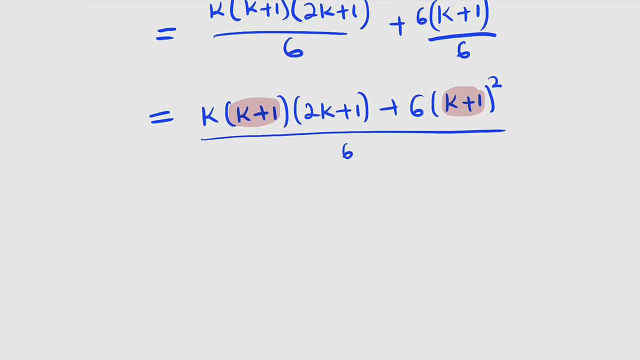 So let us bring it out: If you bring k plus 1 outside Inside, we are going to have k multiplied by 2k plus 1 left From the left hand side. If you multiply k by 2k, you are going to obtain 2k squared. 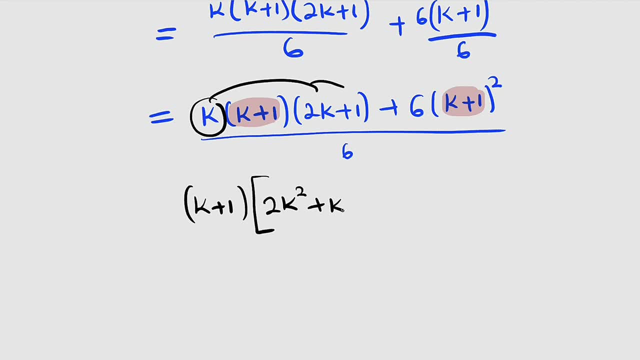 k multiplied by 1 will give us k. And to the other term. You know this is double. 1 is already out. We have k plus 1 left, multiplied by 6.. 6 times k will give us 6k. 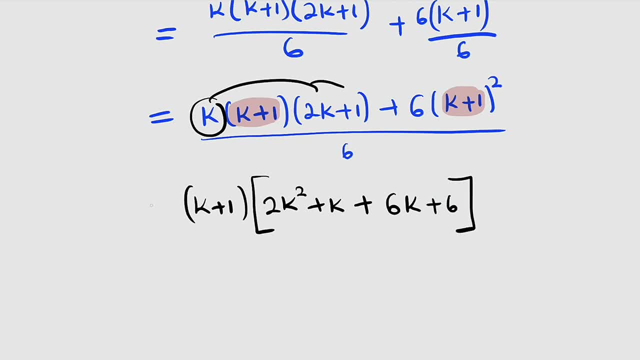 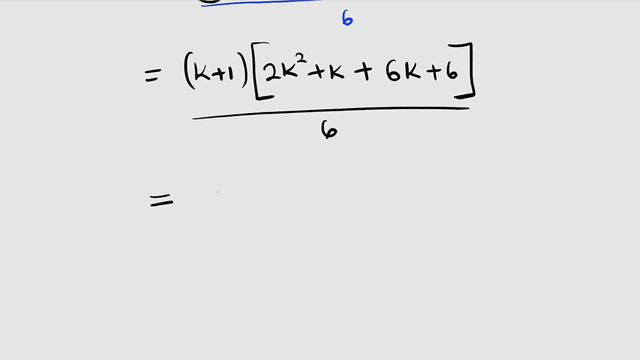 6 times 1 will give us 6.. Remember, the whole of this should be divided by 6.. If you further break it down, You have k plus 1 multiplied by 2k, squared plus 7k, Then plus 6.. 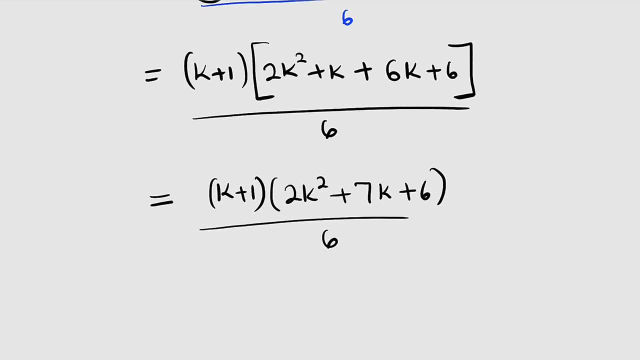 The whole of this divided by 6. The quadratic expression here can be factorized. We are going to take the leading coefficient here And multiply by 6. Which is equal to 12.. Then we think of two numbers which can be multiplied together to get 12.. 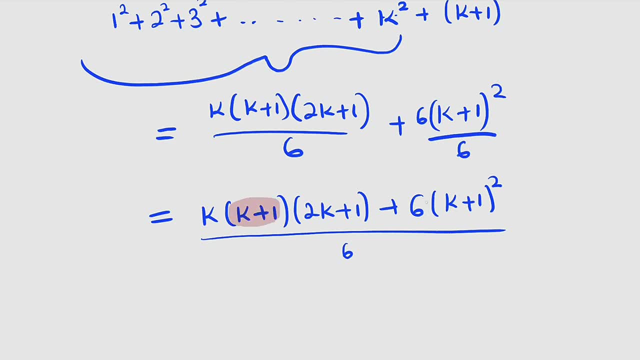 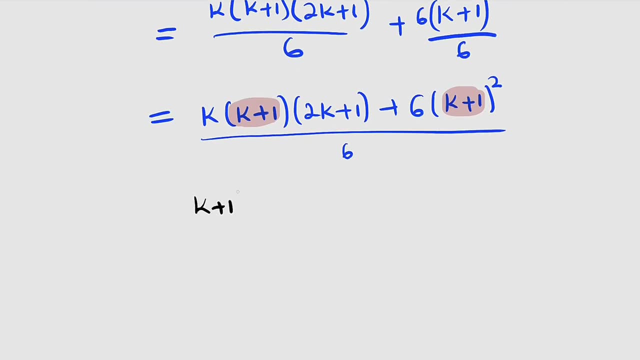 Now, what we have to the top can be factorized because we have k plus 1 in common. So let's bring it out. If you bring k plus 1 outside, Inside we're going to have k multiplied by 2k plus 1 left for the left hand side. 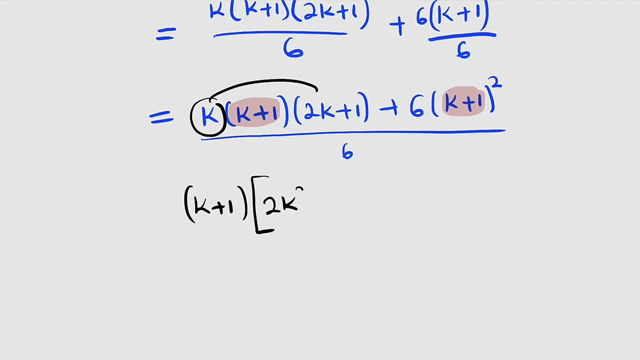 If you multiply k by 2k, You're going to You're going to obtain 2k. squared k multiplied by 1 will give us k And to the other term. You know this is double. 1 is already out. 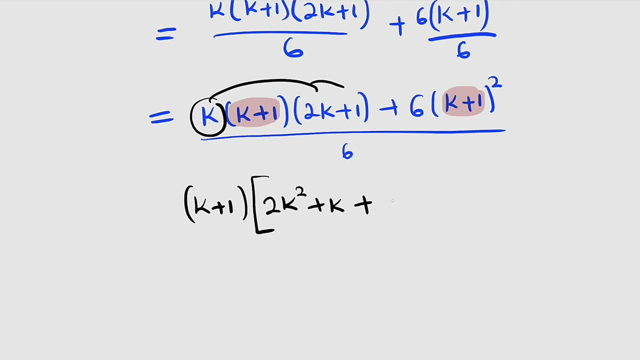 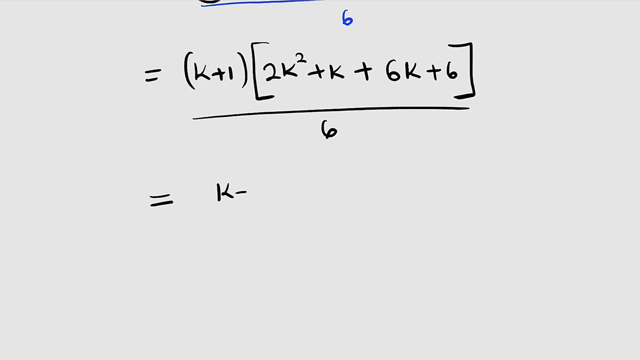 We have k plus 1 left, multiplied by 6.. 6 times k will give us 6k. 6 times 1 will give us 6.. Remember the whole of this should be divided by 6.. If you further break it down, you have k plus 1.. 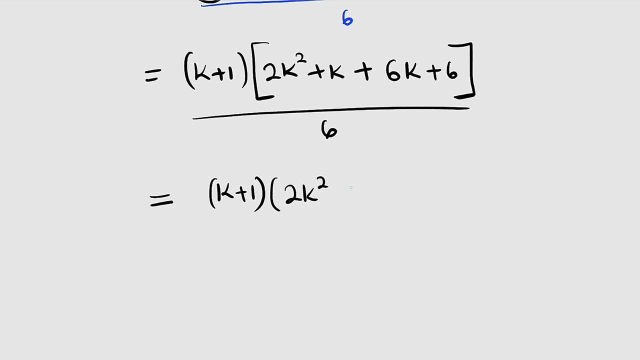 Multiplied by 2k, squared plus 7k, then plus 6, the whole of this divided by 6, the quadratic expression here can be factorized. we're going to take the leading coefficient here and multiply by 6, which is equal to 12. then we think of two numbers which can be multiplied together to get 12 and act together to get the coefficient of k, which is 7.. 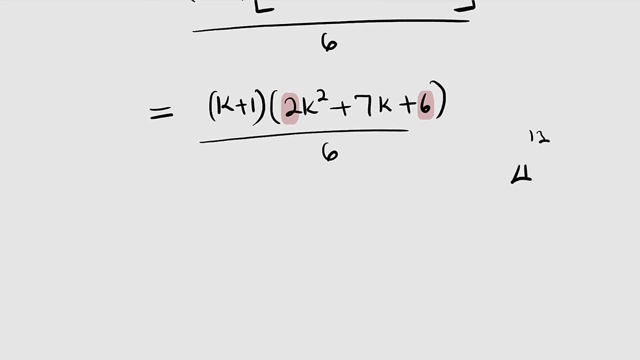 The numbers are 4 and 3.. But since the leading coefficient is 2, we have to divide them by 2.. So these are the numbers we need. We're going to get 2 and 3 divided by 2.. Okay, let's break it down. 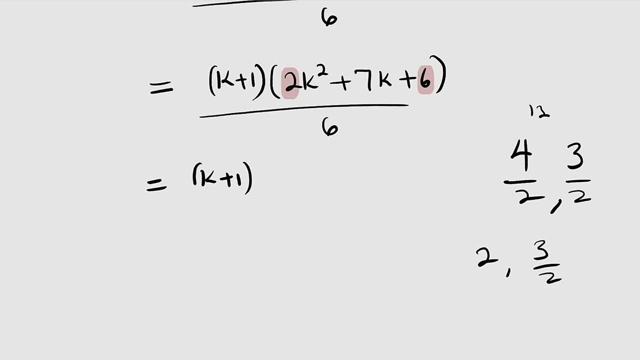 This is equal to k plus 1.. Multiplied by k plus 2.. Multiplied by k plus 3, divided by 2.. But more conveniently we can multiply this and this by 2, so that we have 2k plus 3.. 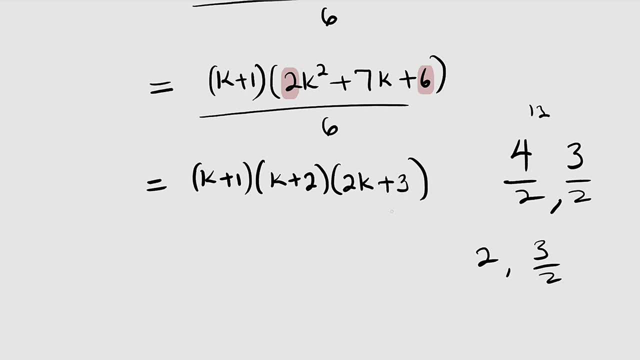 So we have 2k plus 3. The whole of this divided by 6.. So this is what we have to the left hand side, But let us relate it to what we have to the right hand side as well, that they are the same. 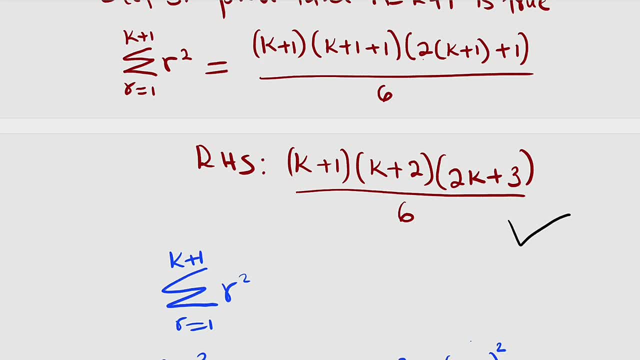 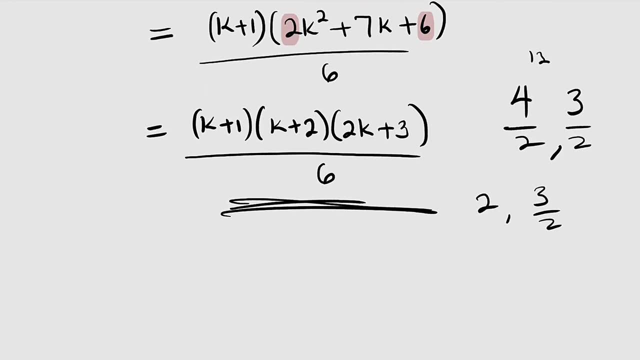 Remember that this is what we have to the right hand side: k plus 1 multiplied by 2.. k plus 2 multiplied by 2.. k plus 3 divided by 6.. And you can see they are exactly the same. So we conclude.